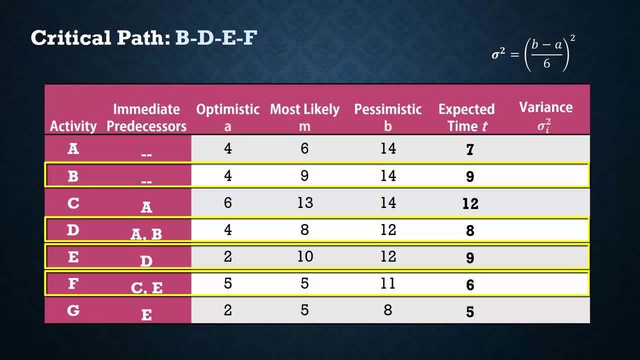 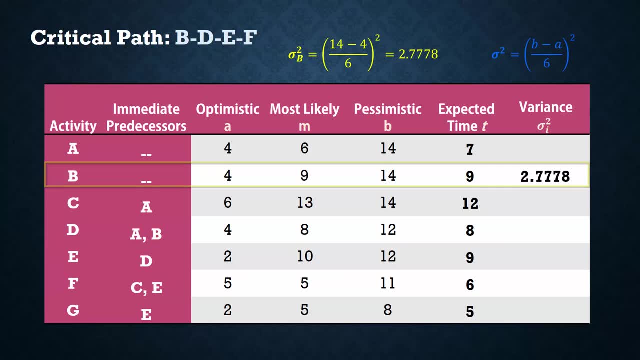 for critical activities. So we only need to calculate the variances for critical activities. Thus, for B, the variance is 2.78.. For D, it is 1.78.. For E, it is 2.78.. For F, the variance is one. 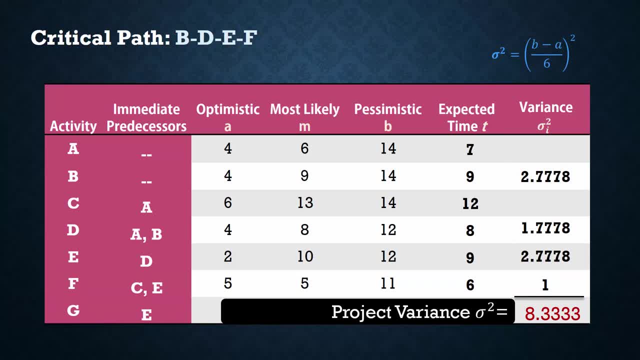 And adding this, we have the project variance of 8.33. Then, taking the square root, we have the project standard deviation of 2.8867.. Note that we have the project standard deviation of 8.33.. Although the uncertainty time estimates are better distributed, 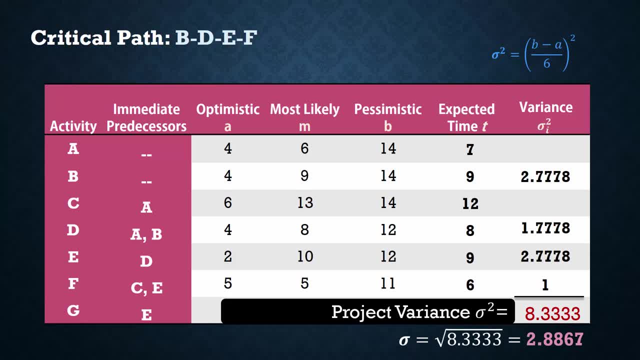 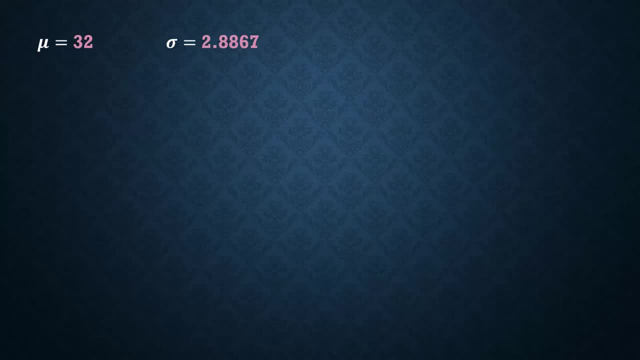 we can approximate the project completion time by a normal distribution With mean equals 32 and standard deviation 2.8867.. So we can apply the Z formula to answer these questions First. we find the probability that the project will be completed within 35 weeks. 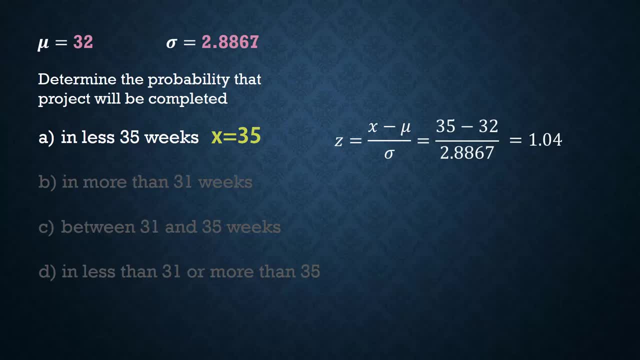 That is X equals 35 and that gives Z equals 1.04.. And looking it up in the tables, we have a less than area of 0.8508.. For X greater than 31, we have Z greater than negative 0.35.. The area less: 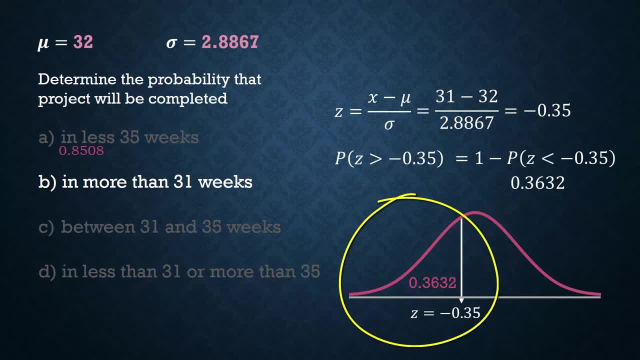 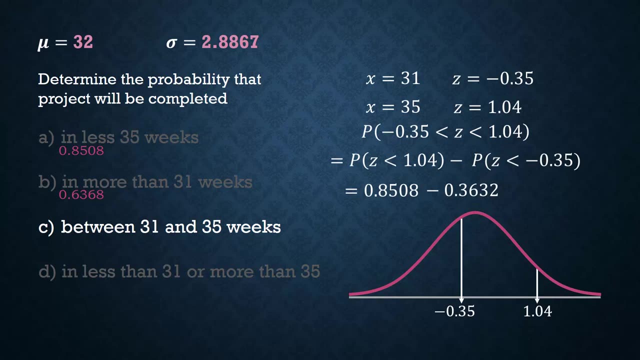 than negative 0.35 is 0.3632.. And subtracting it from 1,, we obtain the more than area of 0.6368.. Between 31 and 35, we find the area between the Z values of negative 0.35 and 1.04 by subtracting. 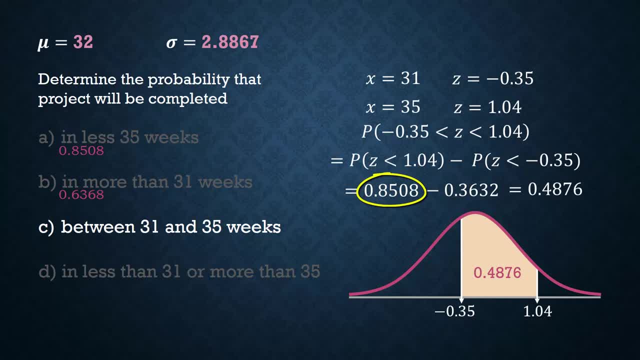 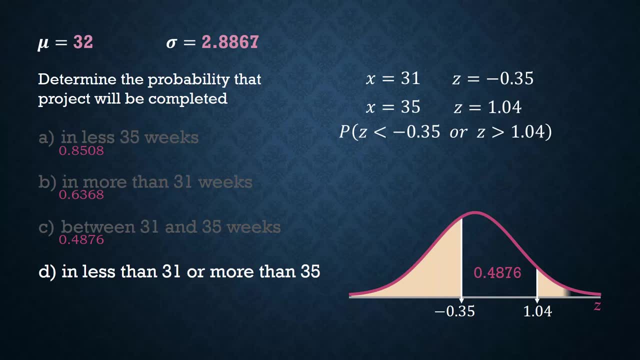 the smaller area of 0.8508.. And looking it up in the tables, we find the probability that the Z value is greater than 0.4876.. For D less than 31 or more than 35 is the complement of our result. 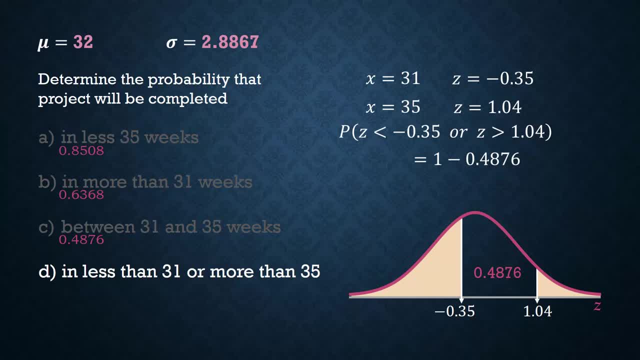 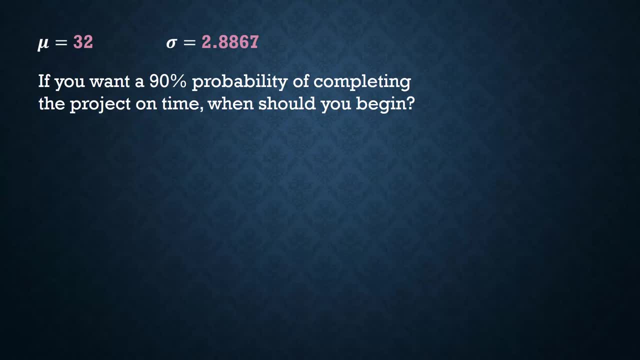 in C. So we just subtract the result from 1 to obtain 0.5124.. Next, if we want a 90% probability of completing the project on time, we do a reverse lookup for a less than area of 0.9.. 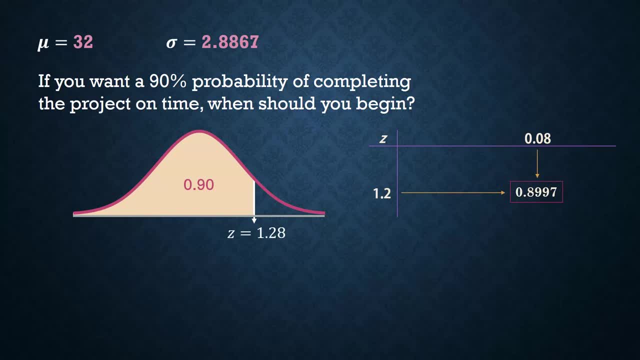 This will correspond to a Z score of 1.4.. And substituting that into the Z formula, we obtain a completion time of about 35.7.. That is, the project should begin about 36 weeks earlier in order to be completed on time.